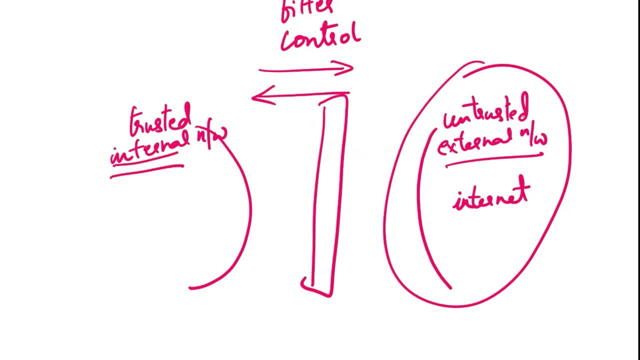 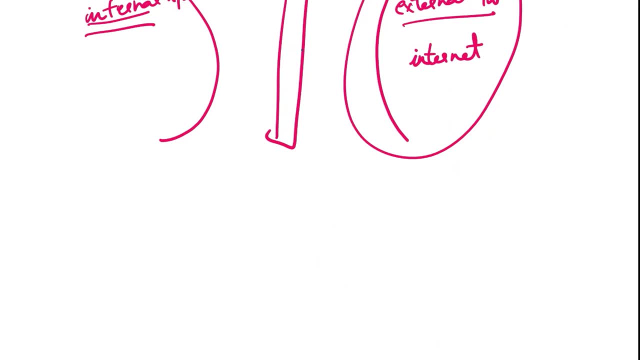 network. This protects the internal network from unauthorized access, cyber threats and malicious activity. Now let's talk about different types of firewalls and their characteristics: their advantages, disadvantages, their use cases. okay, We'll start with the first one, which is packet. 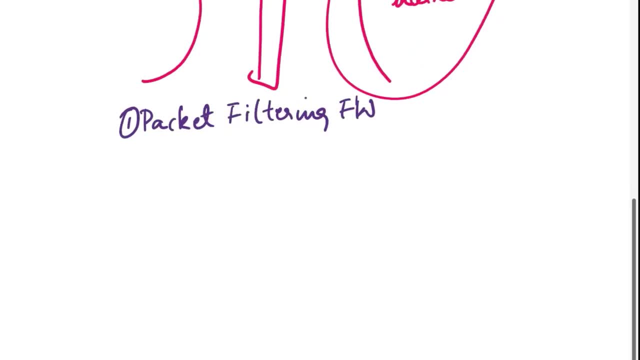 filtering firewall. This firewall is a network security device or software application that operates at the network layer or layer 3.0.. This is a network security device or software application that operates at the network layer or layer 3.0.. This is a network security device or software application. 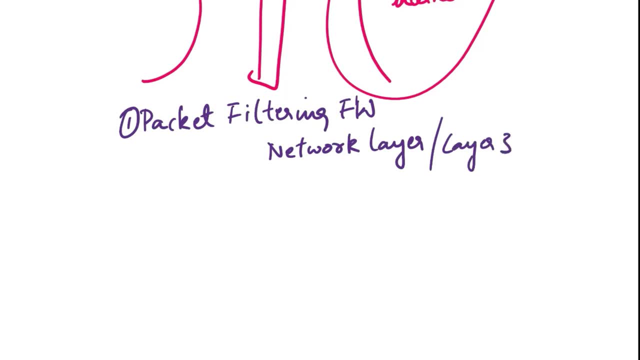 of the OSI model. OSI stands for open systems interconnection- okay, Its primary function is to inspect and control the flow of network traffic based on predefined rules or criteria. These rules or criteria known as ACL, that is, access control lists. okay, These rules determine whether a 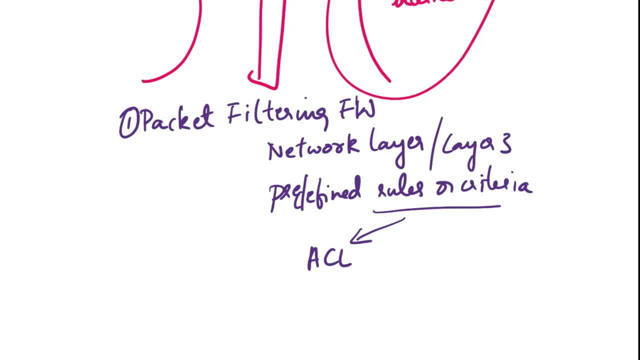 packet should be allowed to pass through the firewall or should be blocked, based on various characteristics of the packet, such as the network security. the network security, the network security, such as source IP address, destination IP address or source port, destination, port and protocol type. Now let's see the characteristics of packet filtering firewall in detail. The first: 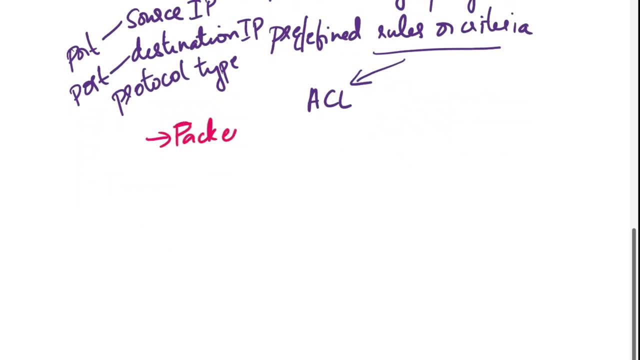 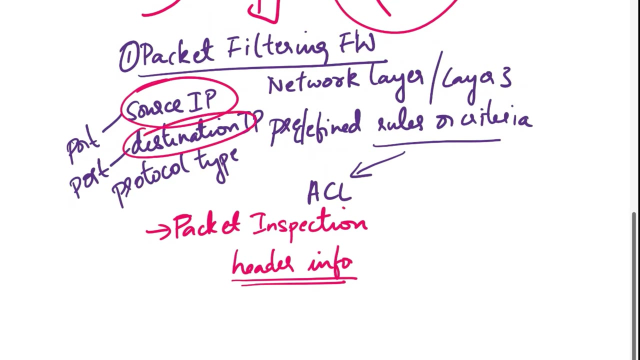 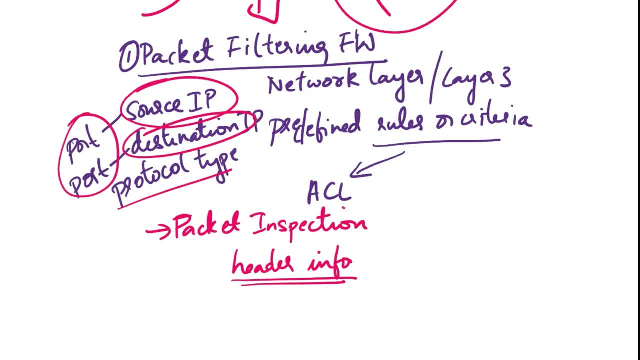 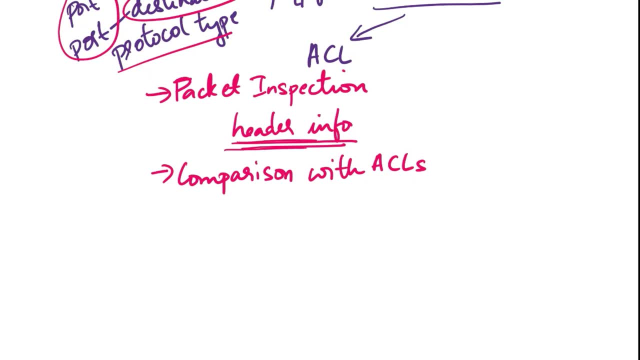 protocol might be TCP, UDP, ICMP, etc. Next characteristic is comparison with the ACLs. The firewall compares the information in the packet header with the rules that are defined in the ACLs, that is, access control lists. These ACLs specify what types of traffic are allowed and what should be blocked. The firewall also compares the information in the packet header with the rules that are defined in the packet header with the rules that are defined in the packet header and sets what type of events and conditions date to be blocked. Next characteristic of packet filtering is: 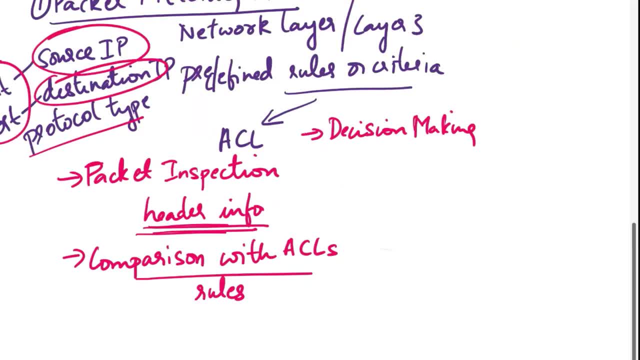 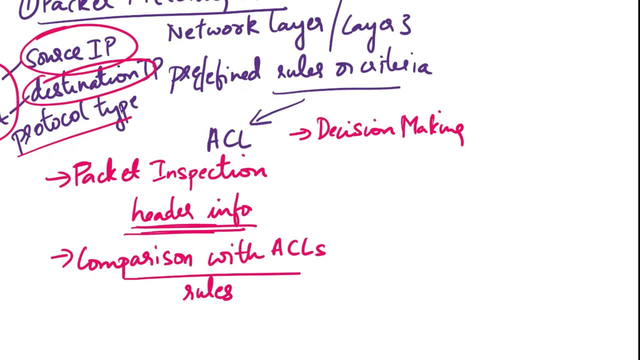 This is 16th- makes decision-making control with application based on the ACL rules. The firewall makes a decision about whether to bu precedence or block the packet If the packet matches on allow rules with ACLs. בא�, heruvitt e and this block rules with ACLs If the acquired a loss of CATLs. 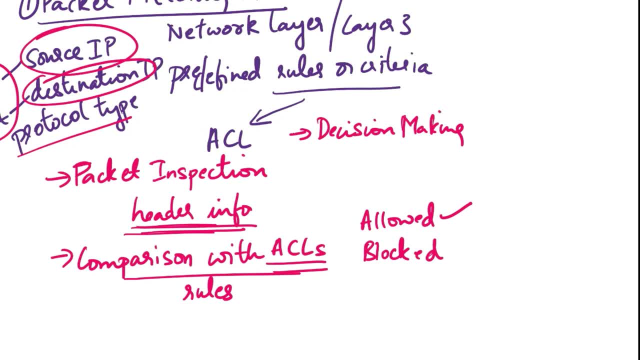 so it is permitted in to buy for the by for this option fast and only by the into the limitation. If it matches a block, the, we will not have bye cd back. the process Next with pick monitoring: Nee, locked rule or doesn't match any rule, then it is either dropped- dropped in the sense, ignored. okay. 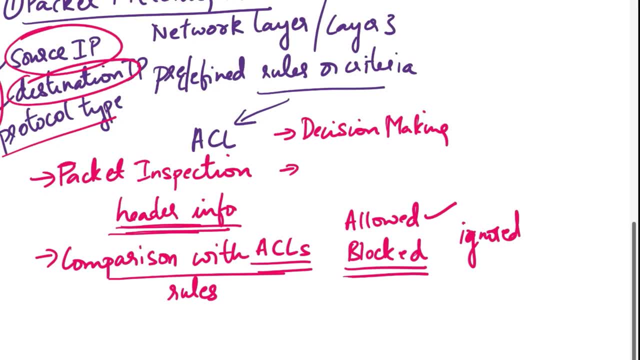 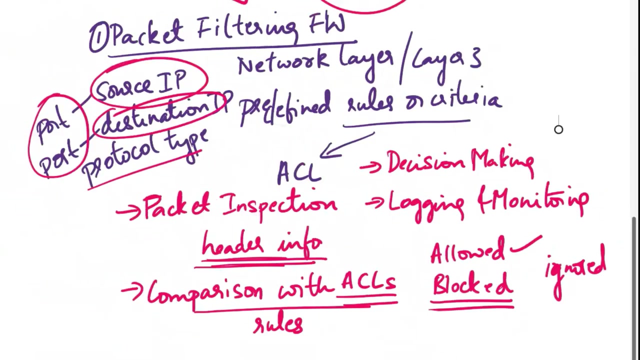 or denied passage. next characteristic we'll be talking is logging and monitoring. many packet filter firewalls provide logging capabilities, allowing the network admins to track and monitor network traffic. this is useful for, like you know, troubleshooting, analyzing security incidents and ensuring that the firewall rules are effectively protecting the network, something that you should. 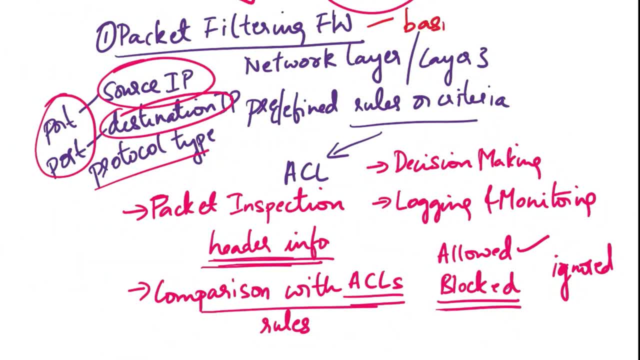 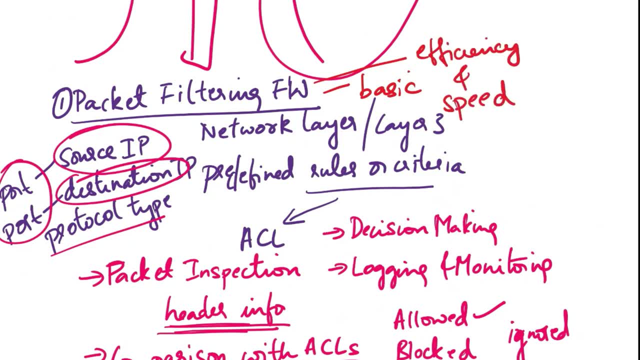 also know is packet firewall is the most basic type of firewall. okay, these firewalls are known for their efficiency and speed in processing network traffic because they operate at a low level in the network stack. that is layer 3, like we said, layer a network layer of the osi. 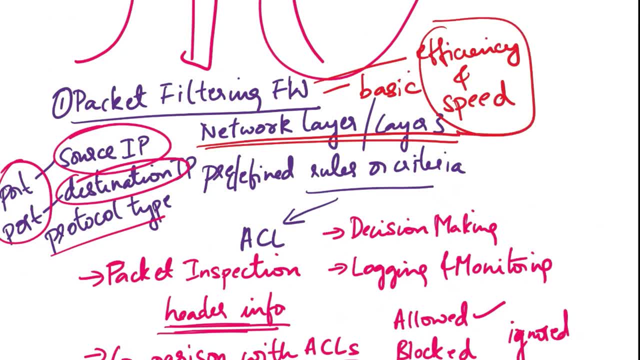 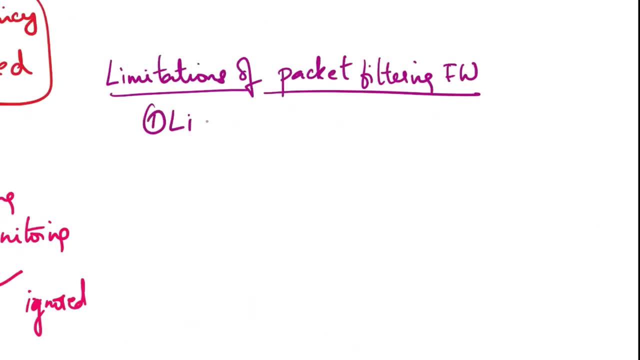 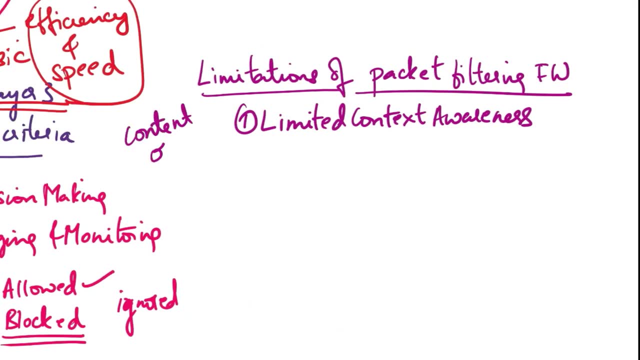 model. even though it provides efficiency and speed, it has some limitations. let's see those limitations, okay. first disadvantage is limited context awareness. packet filtering firewalls do not have the ability to understand the content or context of the data being transmitted. okay, they make decisions solely based on the header. 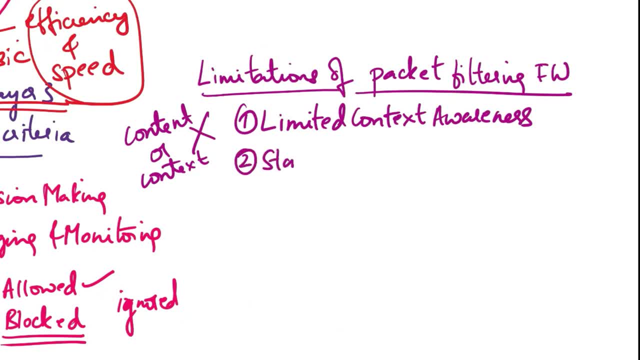 of the packet. next disadvantage is stateless operation. they operate in a stateless manner. that means they do not maintain information about the state of network connections, so they do not have session awareness. this can make them less suitable for handling complex protocols or applications that require session awareness. the 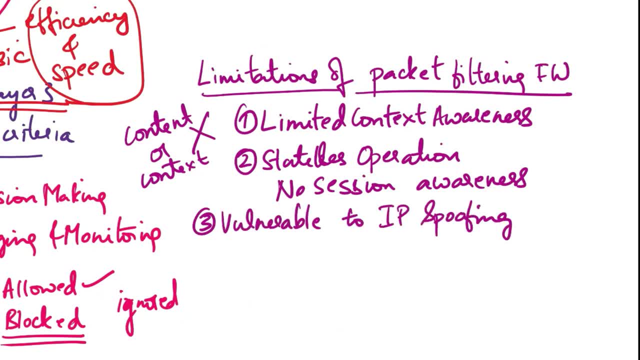 next disadvantage is vulnerable to ip spoofing. packet filtering firewalls can be vulnerable to ip spoofing attacks because they rely on the source ip address in the packet header to make decisions. attackers can force the source ip address to bypass the firewall. despite these limitations, packet filtering firewalls are an 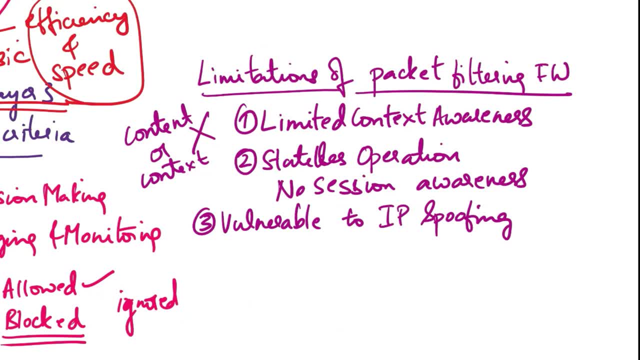 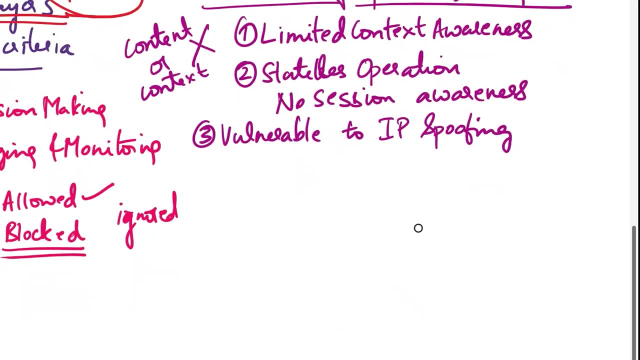 important component of network security and are often used in combination with other security measures, such as intrusion detection system, intrusion prevention systems and application layer firewalls, to provide comprehensive protection for a network. okay, the next firewall type that we'll discuss is stateful inspection firewall. it is also known as stateful. 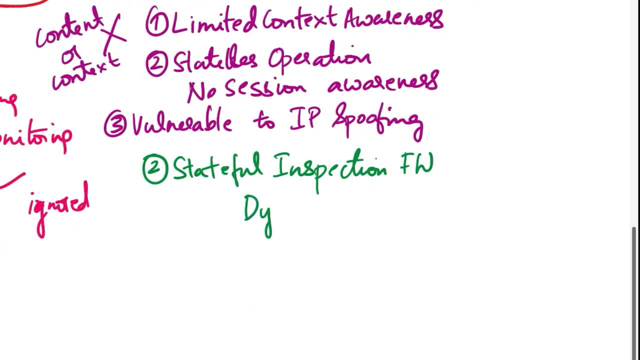 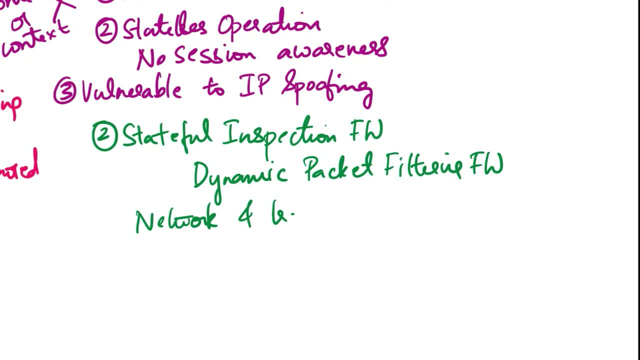 firewall or dynamic packet filtering firewall. this is a more advanced type of network security device or software that operates at the network and transport layers of the osi model. so network layer is at is the layer 3, transport layer is layer 4. okay, in the osi model. so 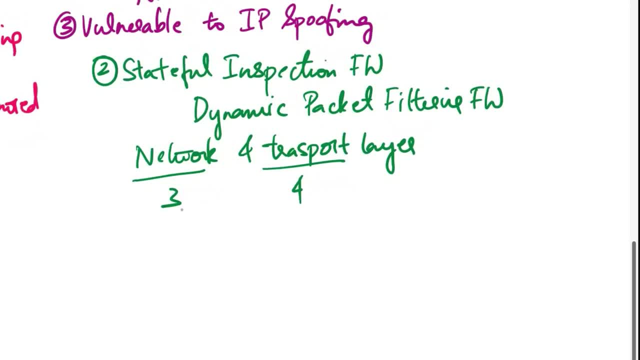 the primary purpose of stateful firewall is to enhance network security by intelligently monitoring and controlling incoming and outgoing network security. by intelligently monitoring and controlling incoming and outgoing traffic, while maintaining an understanding of the state of active network connections. this makes it significantly more sophisticated and effective than basic packet filtering firewalls. let's look. 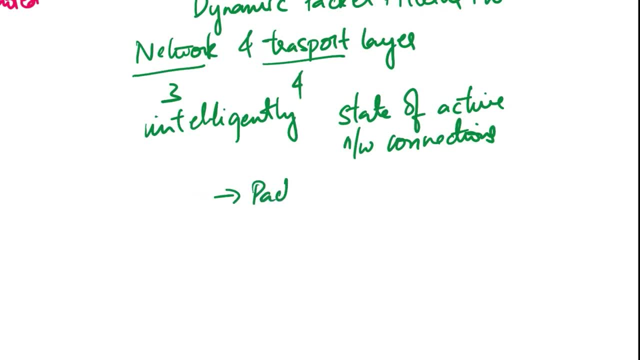 at the characteristics. first one is packet inspection, similar to basic packet filtering firewalls. a stateful inspection firewall examines the headers of network packets to gather information such as source and destination, ip addresses, source and destination, port numbers and the protocol being used. the next characteristic is stateful connections tracking. what distinguishes? 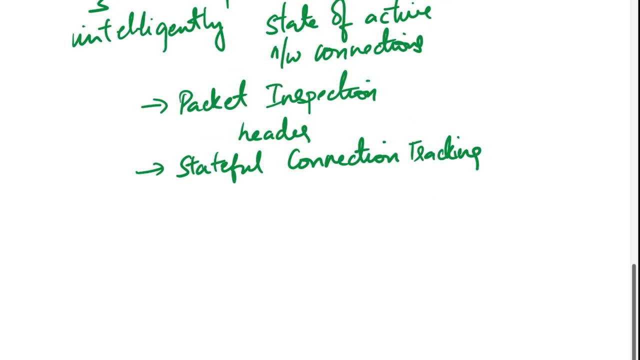 stateful inspection firewalls is their ability to maintain a state table. state table is also referred to, as sometimes you know, connection table or stateful table. this table records the state and details of active network connections. so when a new connection is initiated, the firewall creates an entry in this table, storing information about the connection. 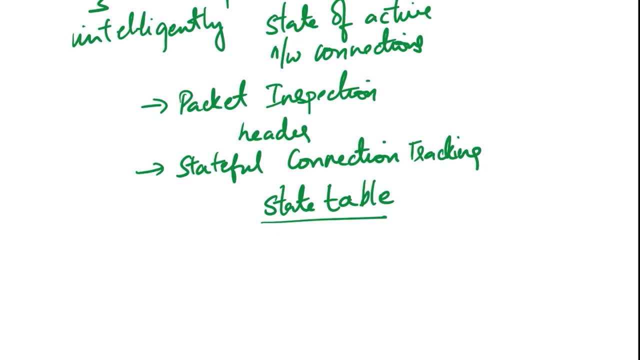 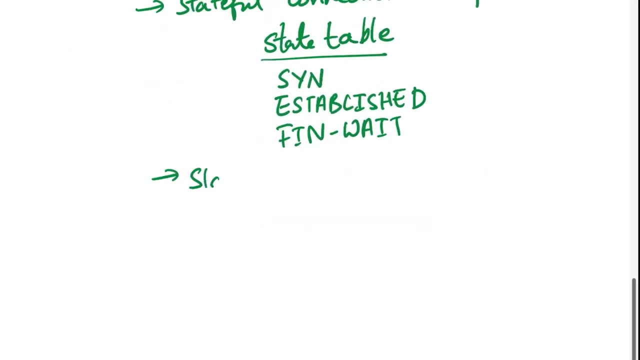 including the source and destination addresses, port numbers and the state of connection. state of connection like can be, like you know, sin connection, established connection, pin weight connection. these are some of the examples and the next characteristic is stateful rule evaluation. as network traffic continues to flow, the firewall continuously. 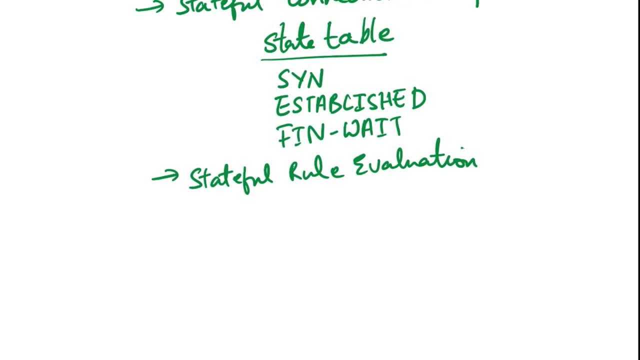 inspects packet headers and compares the information to its state table and predefined access control rules, that is, acls. it takes into account the state information, allowing it to make context aware decisions about whether to permit or deny packets based on the connections established state. next characteristic of the stateful firewall is dynamic rule adaptation. so the stateful 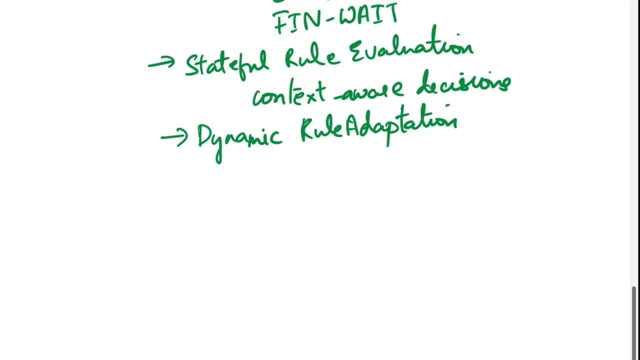 inspection firewall is a stateful rule evaluation. so the stateful inspection firewall is a stateful inspection firewall, an application where system or controller can automatically adjust the network connection status. you can also see the domain and the direct connection to the network and have the data of network connection which can send through the network. 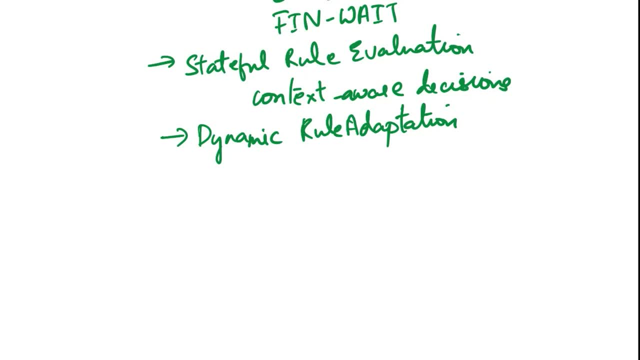 as feedback to the network when you set up functions or other components. for example, once an connection is established, the firewall may allow related inbound traffic without requiring specific rule definitions, since it recognizes the association with an existing legitimate connection. next characteristic is session awareness. since stateful inspection firewalls maintain state information, they possess a level of session. 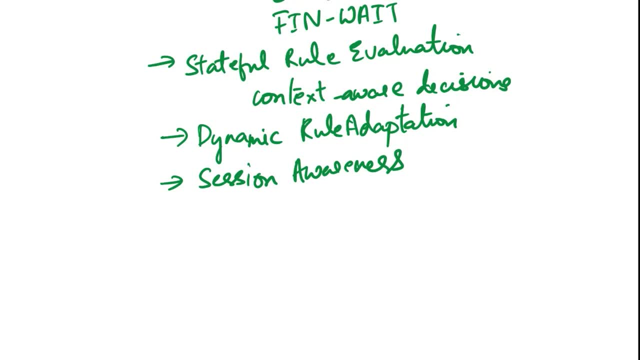 awareness, allowing them to understand the context of network sessions. this enables them to detect and prevent certain types of attacks that involve session manipulation or intrusion attempts within an ongoing session. this provides a higher level of security. the next characteristic is logging and monitoring, like packet filtering firewalls that we discussed, right even the stateful inspection. 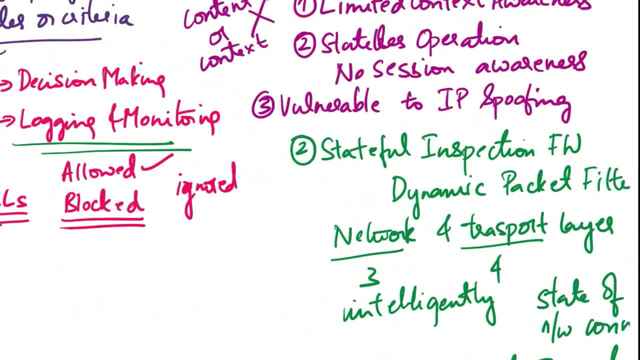 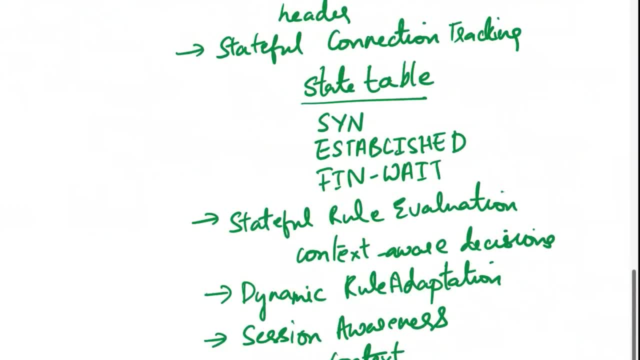 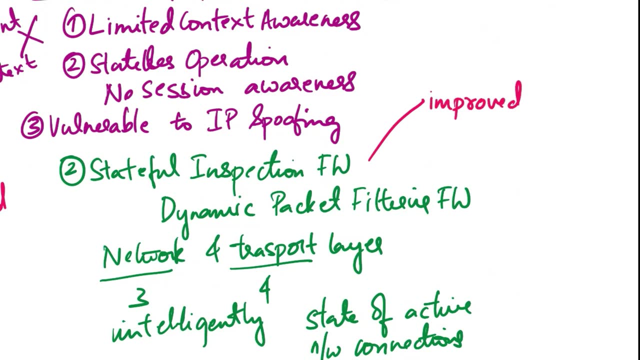 firewall typically offers logging and monitoring capabilities. this allows the network administrators to track and analyze network traffic and security incidents. key advantages of security inspection firewalls include improved security. this is due to their ability to understand the state of network connections and adapt rules accordingly. they are more effective at preventing 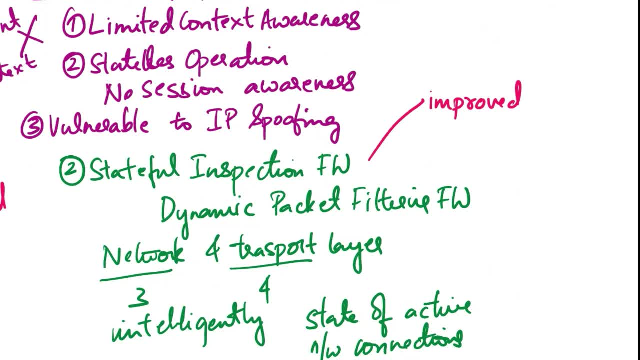 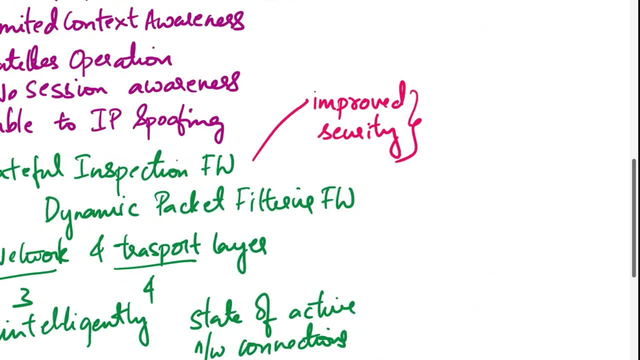 attacks like ip spoofing and various forms of packet level and session level attacks. so improved security is the advantage provided by stateful inspection firewall, but they may introduce some latency in processing traffic compared to basic packet filtering firewalls, due to the additional state tracking and rule evaluation. stateful- 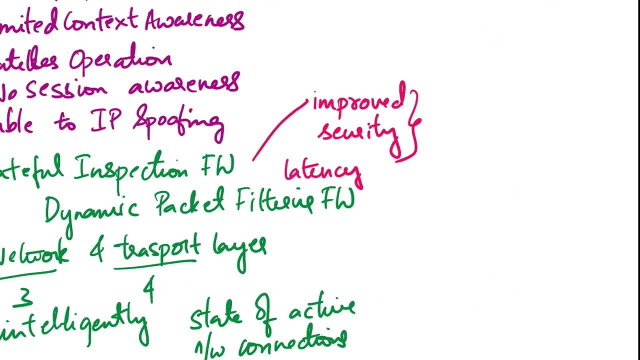 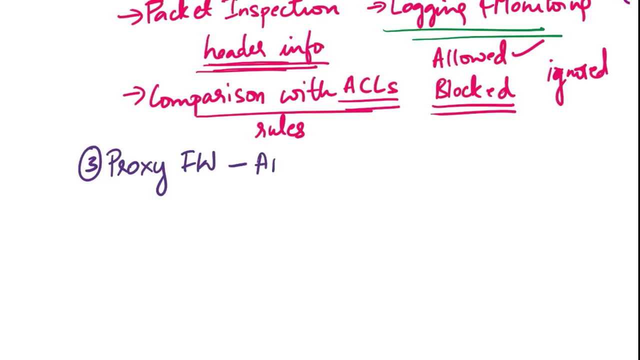 inspection firewalls are commonly used in modern network security architectures and play a crucial role in protecting enterprise networks from sophisticated threats. okay, the next type of firewall that we'll discuss is proxy firewall. this is also known as application layer firewall, or sometimes as application proxy firewall. this is a type of 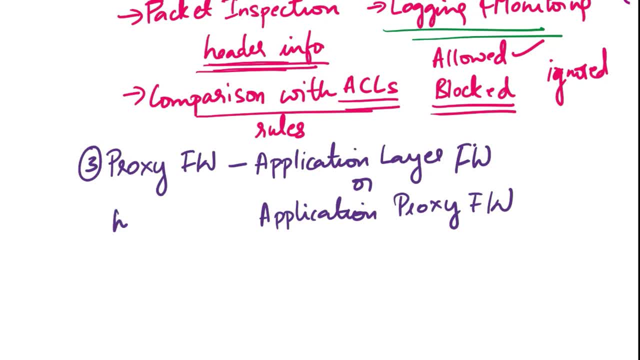 network security device or software that operates at the highest osi layer, that is, layer 7 or application layer. so we learn that packet filtering firewalls and stateful inspection firewalls operate at lower network level. so this is a type of network security device or software that operates at the highest osi layer. we are observing a 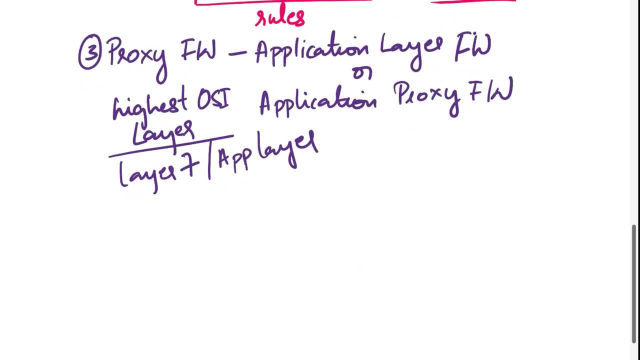 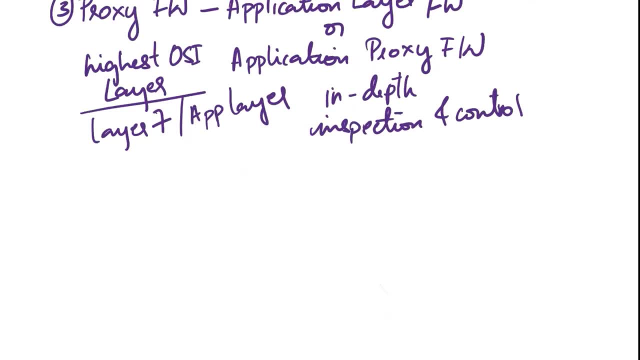 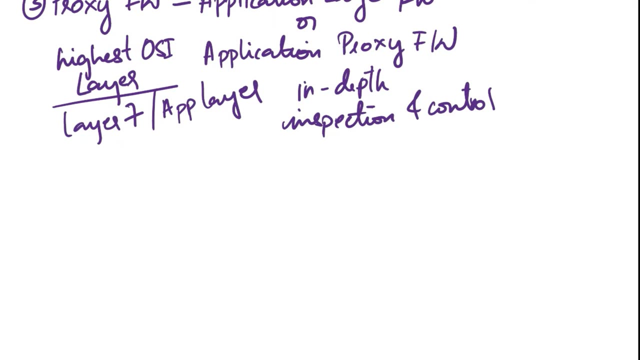 levels. right proxy is at the highest level and proxy firewalls are designed to provide in-depth inspection and control of network traffic. at the application layer, they act as intermediaries between clients and servers, effectively serving as the gateway for application level traffic. so let's see the characteristics in more depth. the first characteristic is intermediary role. 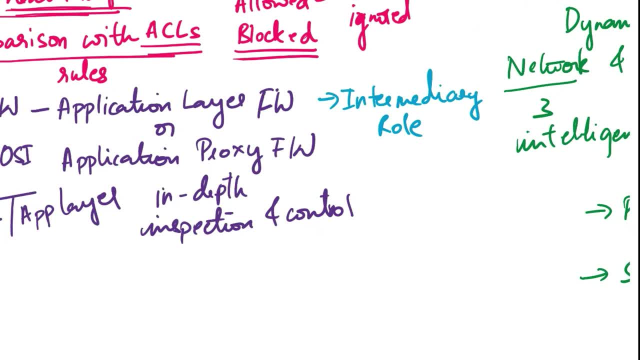 like i mentioned before, proxy firewalls inspect and handle traffic on behalf of client devices. when a client wants to access a remote server, it sends its request to the proxy firewall instead of directly communicating with the server. the next characteristic is app layer inspection. unlike lower level firewalls that only examine packet headers, proxy firewalls perform deep. 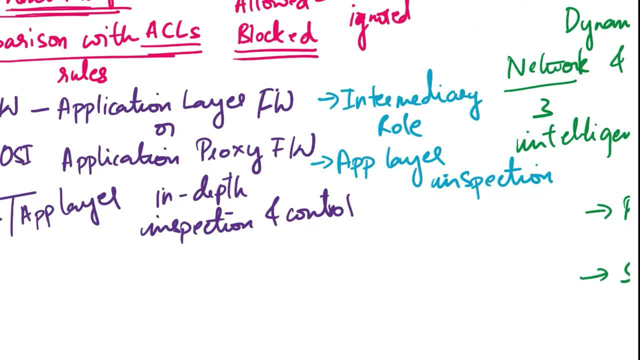 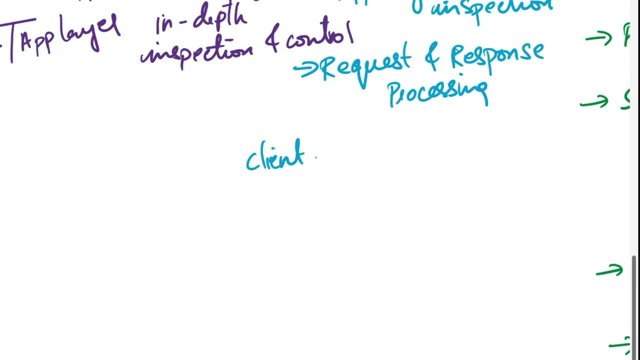 packet inspection at the application layer. this means they can inspect and analyze the content, protocols and behaviors of specific applications. next characteristic is request and response processing. so there is a client, like i mentioned. the client sends the request to the proxy firewall instead of the server. so when 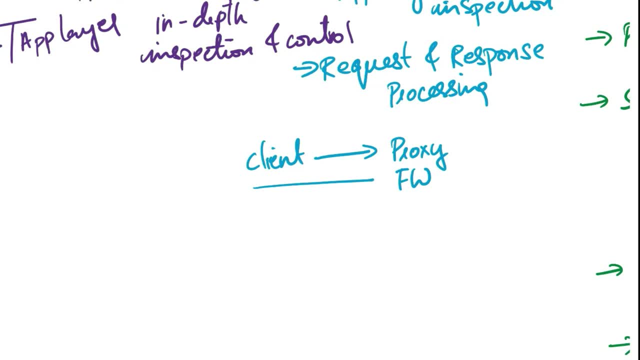 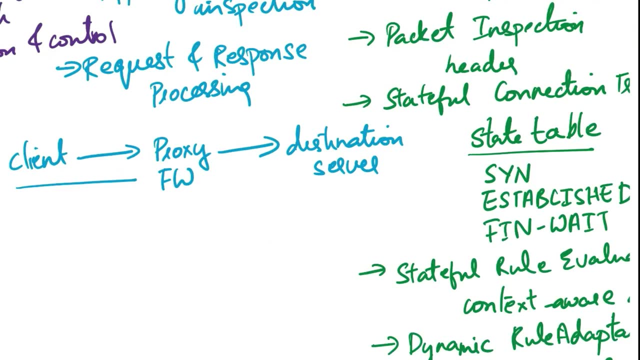 a client sends a request to the proxy firewall, the proxy firewall forwards the request to the destination server, and this is for the client to send the request to the destination server. the client is forwarding on behalf of the client, right? the firewall then receives the server's response. so this is the request, that is, it is sending and it is getting a response from the. 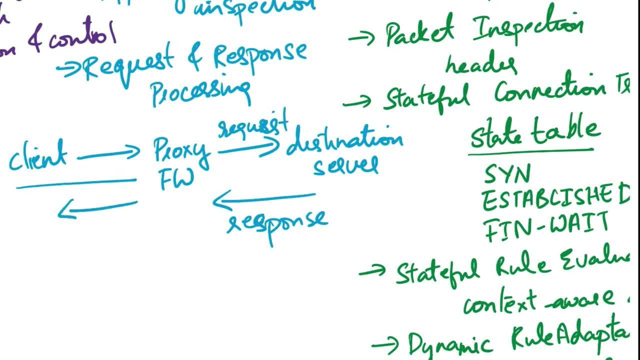 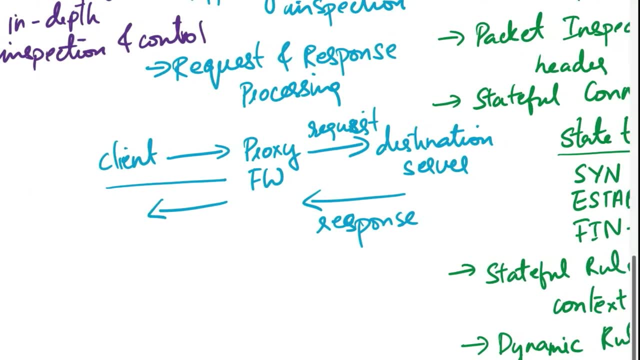 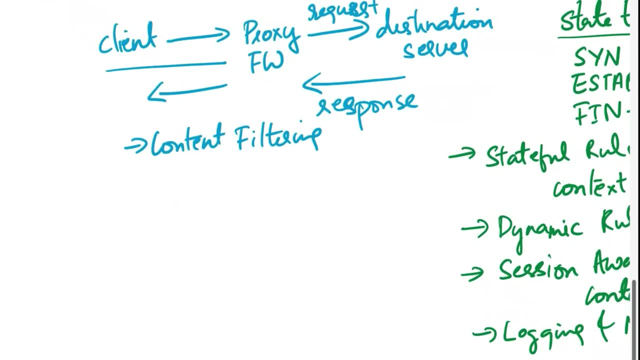 server and then it sends it back to the client. this process involves parsing and understanding the application layer data in both the request and response. the next characteristic is content filtering. proxy firewalls, or app layers, are the second characteristic of a proxy firewalls. Application firewalls enforce granular access control policies based on application specific. 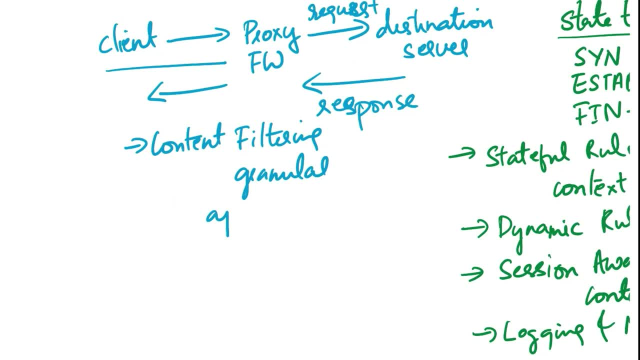 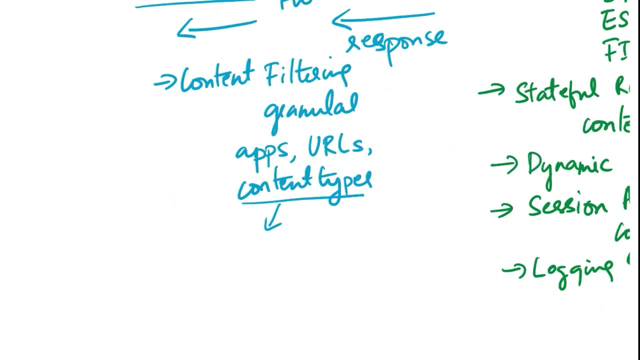 criteria. They can allow or block specific applications, URLs, content types. like you know, content type can be in the companies. you can block entertainment like Netflix. you're blocking everything, And these firewalls even provide specific features within the applications to be blocked. 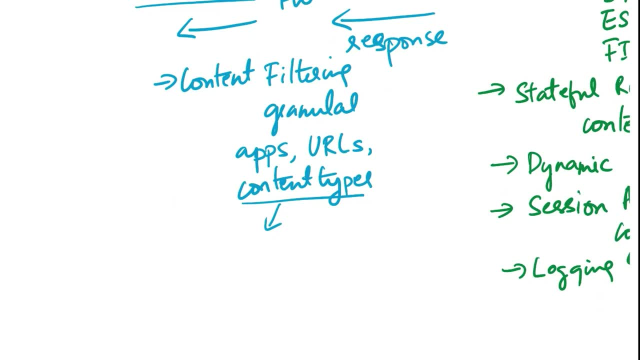 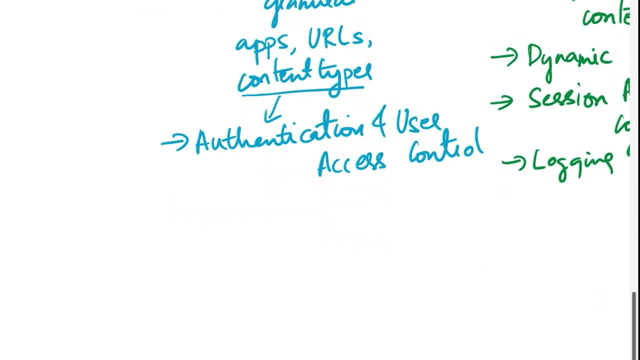 Like, suppose say, blocking file uploads on social media sites. Okay, the next characteristic is authentication and user access control. Many proxy firewalls support user authentication, which means users must log in before accessing the internet or specific applications. This allows organizations to enforce user specific policies and track user activity. 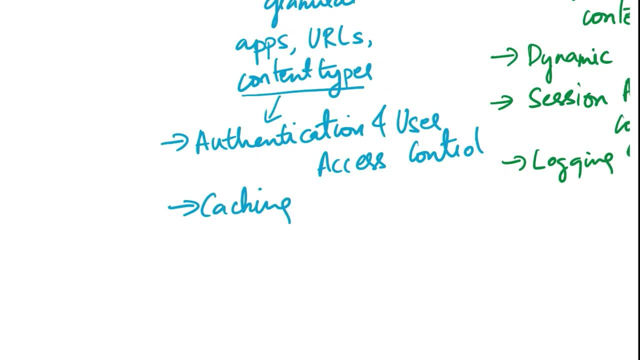 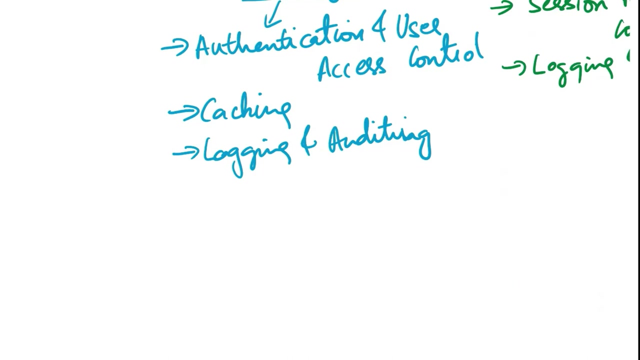 And the next characteristic is caching. Proxy firewalls often include caching capabilities to store frequently accessed content locally. This can improve network performance by reducing the need to fetch the same content repeatedly from remote servers. Next is logging and auditing. Proxy firewalls maintain detailed logs of user activities and application traffic. 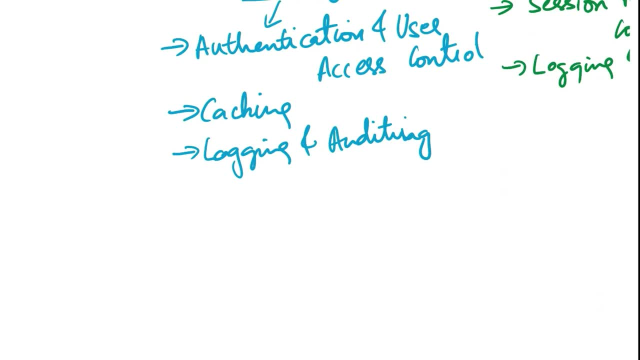 This information is valuable for security monitoring, compliance and forensic analysis. And the next characteristic is security and privacy. Proxy firewalls can provide an additional layer of security by isolating the internal network from external threads. They can also enhance user privacy by masking client IP addresses from external servers. 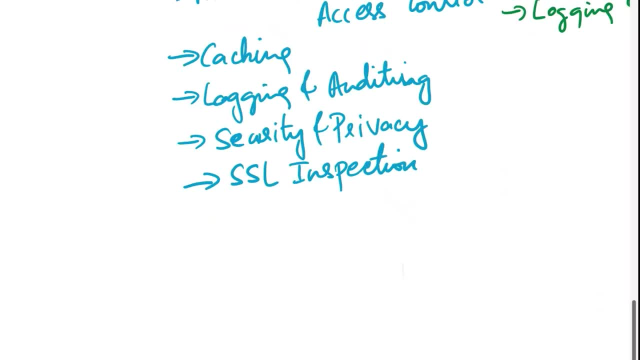 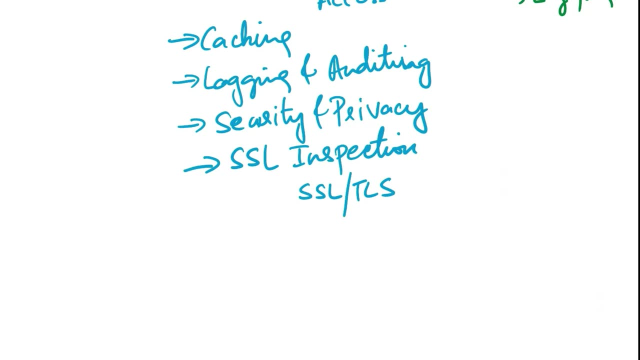 Next one is SSL inspection. Some proxy firewalls support SSL and TLS inspection, allowing them to decrypt and inspect the data, And they can also detect encrypted HTTPS traffic for potential threats or policy violations. So proxy firewalls are often used in environments where granular control over internet usage and application access is required. 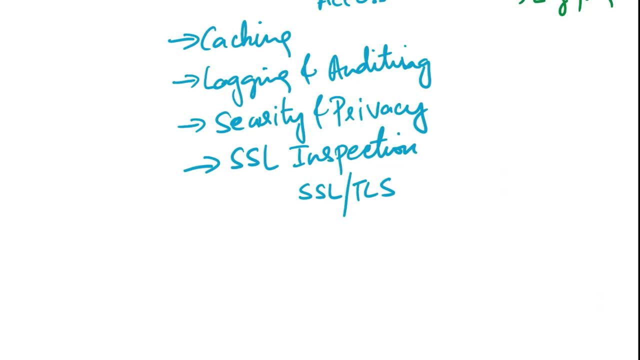 such as corporate networks, educational institutions and government organizations. They are effective at protecting against various web-based threats, managing bandwidth usage and ensuring compliance with security and privacy and usage policies. So, even though it provides so many advantages, proxy firewalls can introduce. 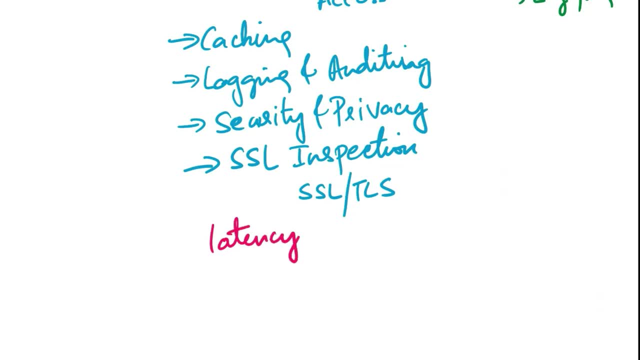 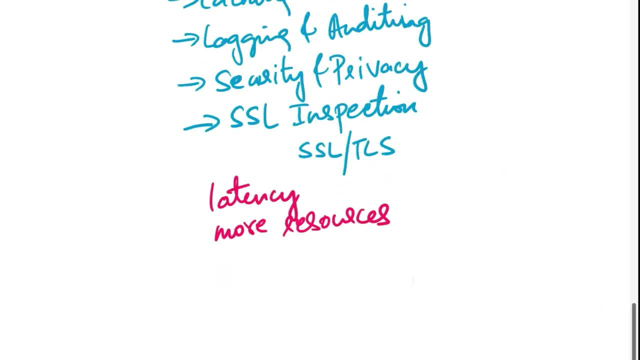 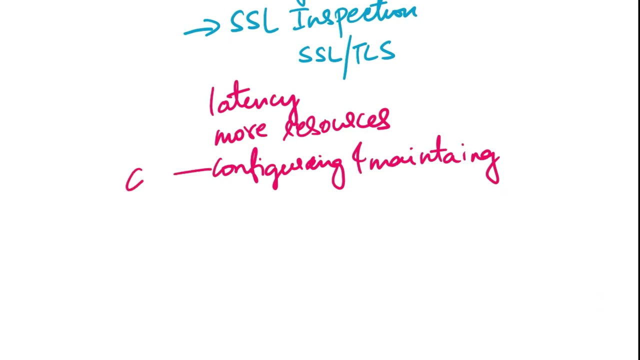 some latency due to the additional processing involved in handling application layer traffic, and they may require more resources compared to lower level firewalls. Additionally, configuring and maintaining proxy firewalls can be complex. This is especially true when you are handling larger networks with diverse application requirements. The next firewall type that 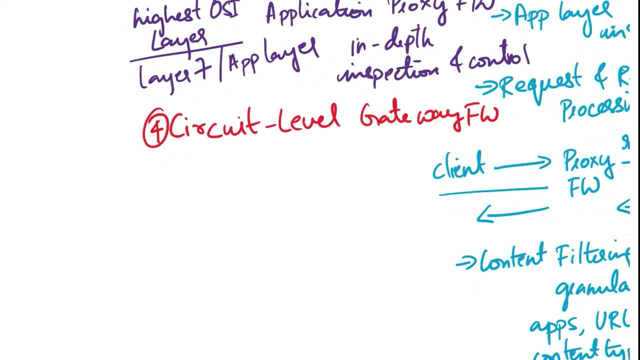 we'll discuss is circuit level gateway firewall. This is also known as circuit level proxy or a circuit level firewall. It is a network security device or software that operates at the session layer of the OSI model. Session layer is layer 5.. Unlike the application layer firewall, which 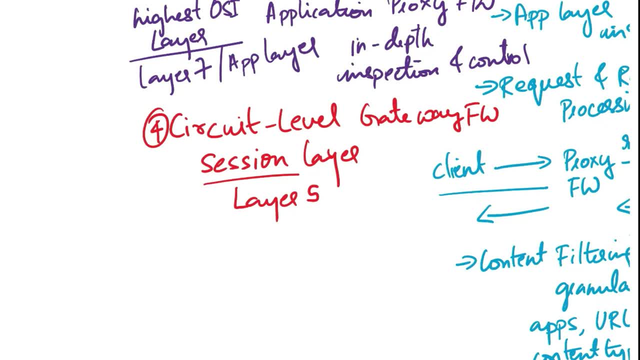 works at the application layer to inspect and filter. it is a network security device. Application specific data circuit level gateways focus on the session level control of network traffic, particularly for TCP connections, that is, transmission protocol connections. Let's look at the characteristics in more depth. First one is, like we mentioned, session level control Circuit. 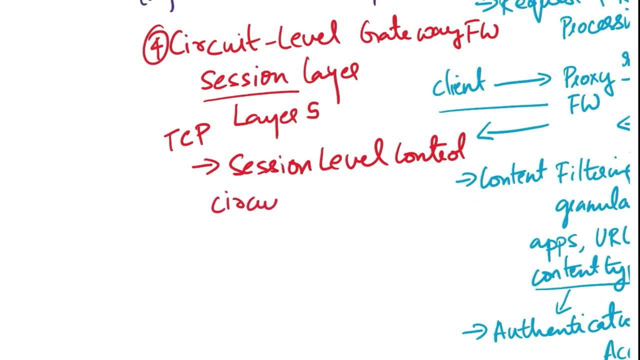 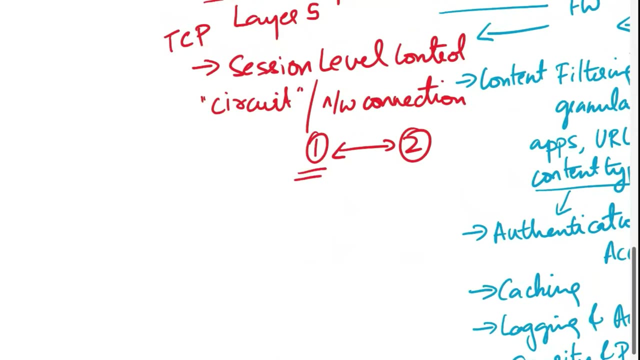 level gateways work by creating a circuit or network connection between two hosts. So this is host one, this is host two, this is host three, this is host four, this is host five, this is host six and this is host seven and this is host eight. So one host is inside a protected network. 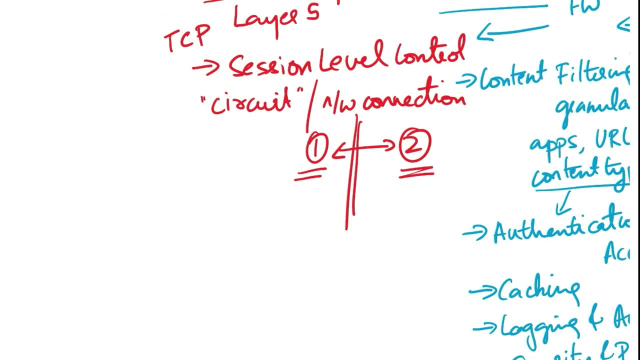 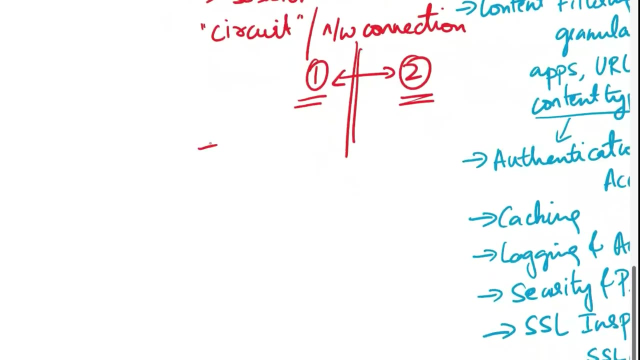 and the other one is outside a protected network. These gateways do not inspect actual application layer data like HTTP requests or FTP commands, but focus on the establishment and management of network sessions. Next characteristic that we will discuss is proxying network connections. So say, there is a client, this client is inside a protected network and this initiates a connection. 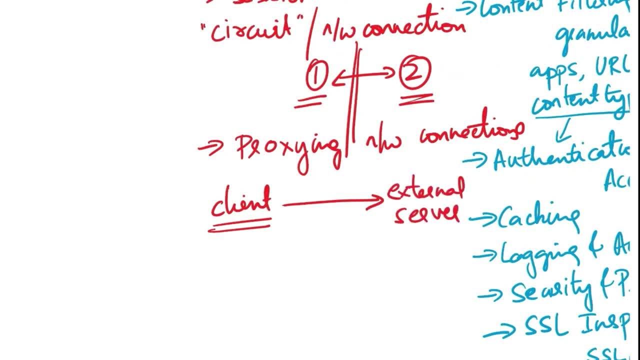 with an external server. When this connection is initiated, network circuit gateway acts as a proxy by creating a separate connection to the external server on behalf of the client. So this means that the external server sees the circuit level gateway as the source of the connection and not the 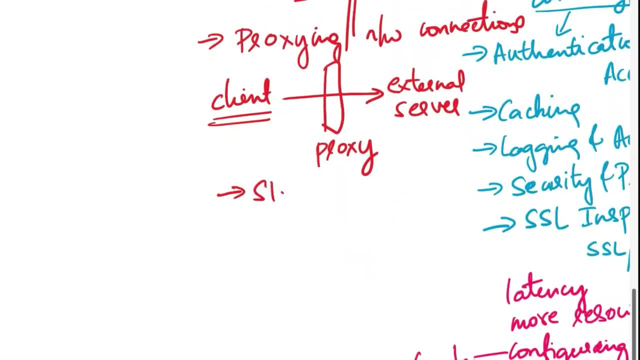 internal client. Next characteristic is stateful inspection. Circuit level gateways maintain a state table that tracks the status of network sessions, primarily for the TCP connections. This allows them to monitor the state of TCP sessions, such as whether they are in the process of being established, or they are established or closed. Next characteristic is related to the 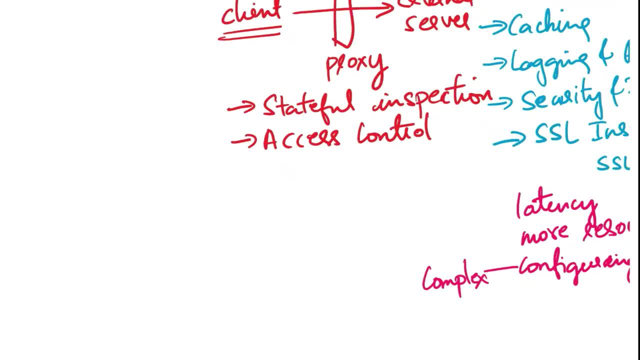 access control. They can enforce access control policies. This is based on source and destination IP addresses, port numbers and session level attributes. For example, you can configure rules to allow or deny certain hosts or networks from establishing specific types of TCP connections. The next characteristic is related to NAT, that is, 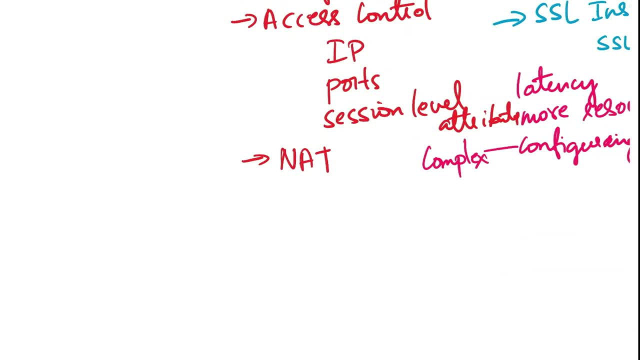 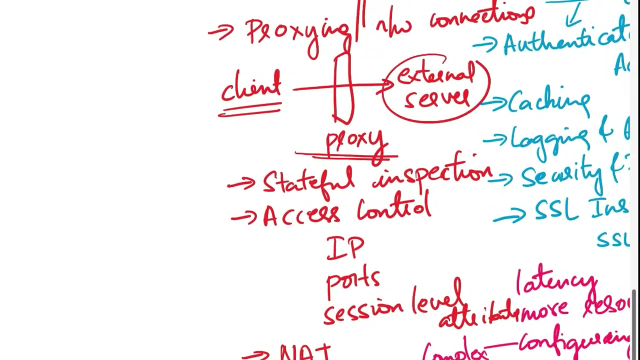 network address translation Circuit level gateways may perform NAT, which involves changing the source or destination IP addresses. This is based on source and destination IP addresses And port numbers to obscure the internal network structure from external hosts. NAT can enhance security and privacy, Like we said here right while discussing proxy, that the external server 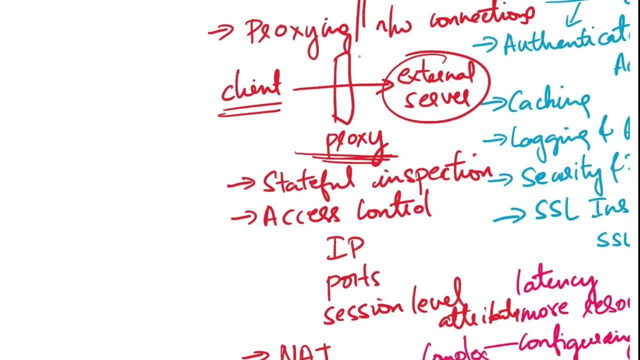 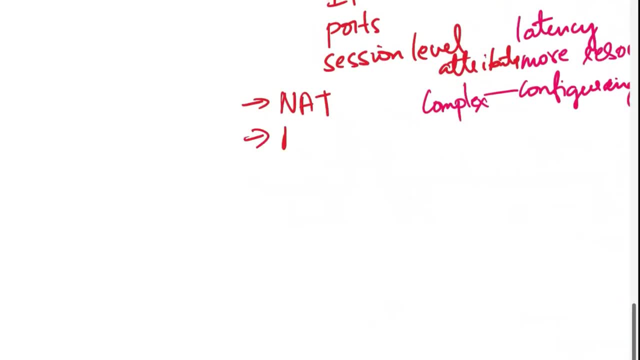 can see only the proxy, in the sense the gateway, circuit level gateway, and not the client. The next characteristic is application agnostic. Unlike application layer firewalls, circuit level gateways are application agnostic. They do not examine the content of data being transmitted. 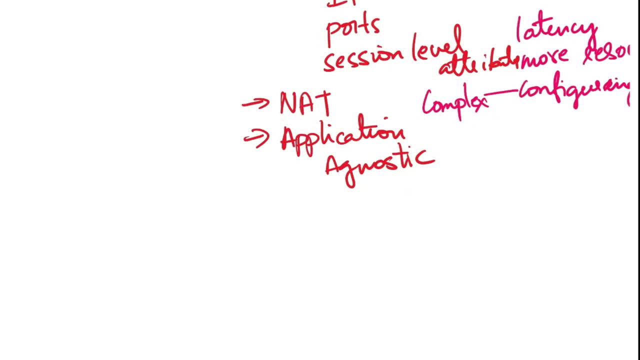 making them suitable for scenarios where only session level control and basic network protection are needed. Circuit level gateways are often used in situations where a high level of network connectivity is required, but detailed inspection of application data is not necessary or may not be desirable, For example. 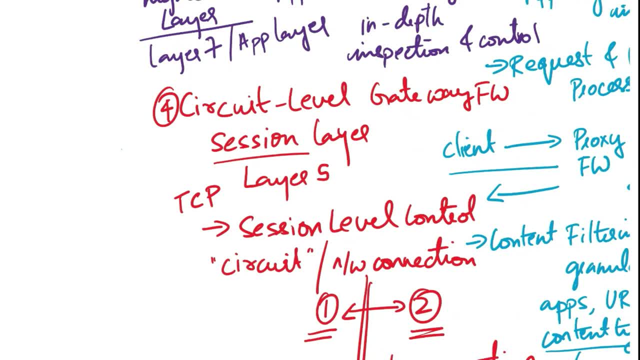 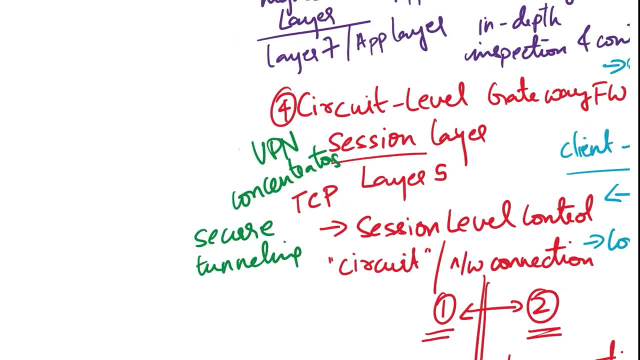 are very commonly used in. For example, they are commonly used in VPN concentrators and in scenarios where secure tunneling or connectivity between networks is essential. While circuit level gateways provide certain benefits, such as network level security and the ability to obscure internal network details, they have limitations too. First is they do not provide granular application level. 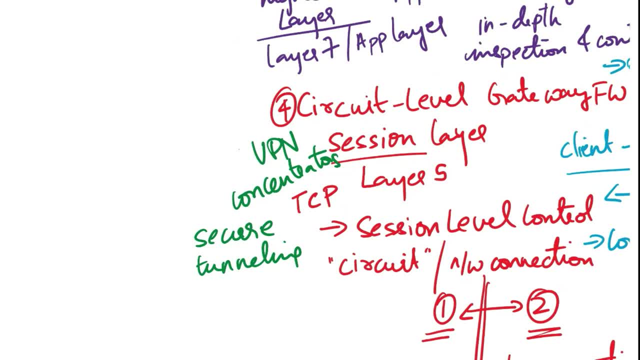 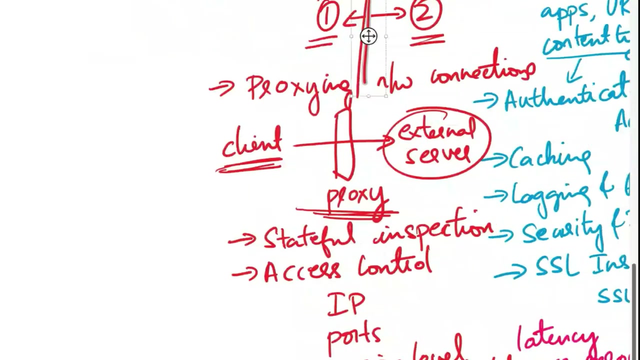 control or content filtering, making them less suitable for enforcing application-specific security policies. For comprehensive security, organizations often use circuit level gateways in conjunction with other security measures such as application layer firewalls or intrusion detection or prevention systems. The next firewall type that we will discuss is next generation. 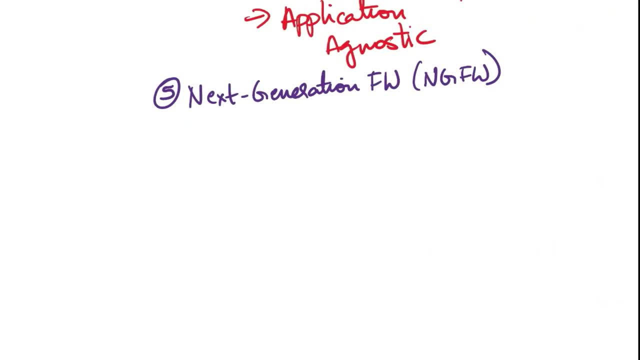 firewall. A next generation firewall is a sophisticated network-based and secure network security system that can be used to secure network security devices, or software that combines the capabilities of traditional firewalls with advanced features to provide a comprehensive and multi-layered security for modern network. 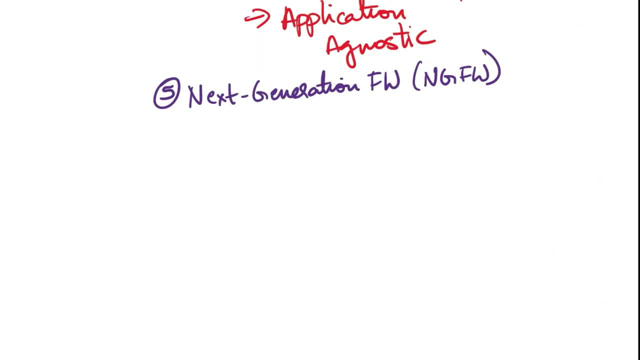 environments. These firewalls are designed to address the evolving threat landscape and the complex network traffic patterns associated with today's IT infrastructure. They operate at multiple layers of the OSI model, including layers 3,, that is the network layer, layer 4,, that is the transport layer, and layer 7,, which is the 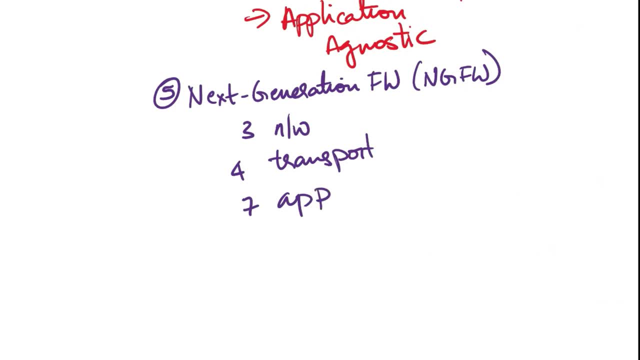 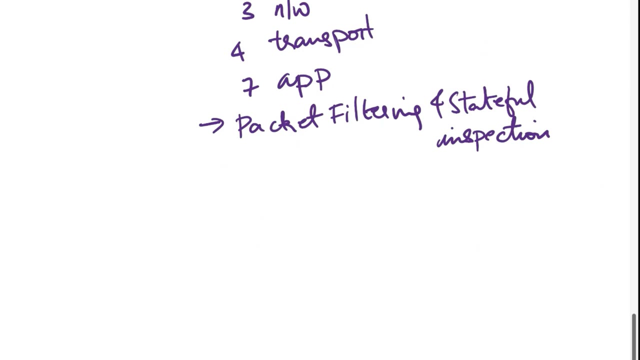 application layer and offer several key features and functionalities. Let's see a few of them. The first one is packet filtering and stateful inspection. Like traditional firewalls, next generation firewalls perform packet filtering and stateful inspection to analyze and control network traffic based on source and 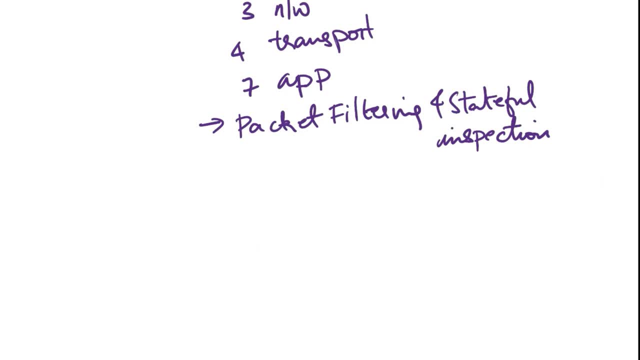 destination IP addresses, port numbers and protocols. This basic level of security helps prevent unauthorized access and basic network level attacks. Next characteristic is application awareness. Next generation firewalls go beyond simple port-based filtering by using deep packet inspection, DPI and application identification techniques to recognize and control applications. 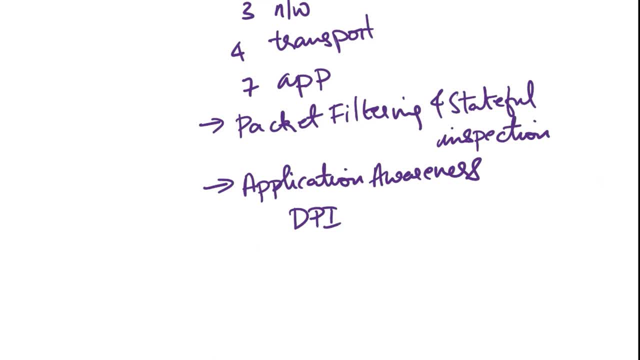 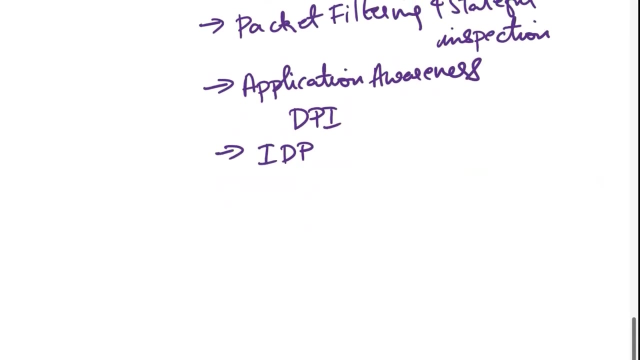 and services running on the network. Next generation firewalls are designed to ensure that the network is protected and secure. This enables them to enforce granular access policies based on specific applications or application categories. Next one is intrusion detection and prevention. Next generation firewalls often incorporate intrusion detection. 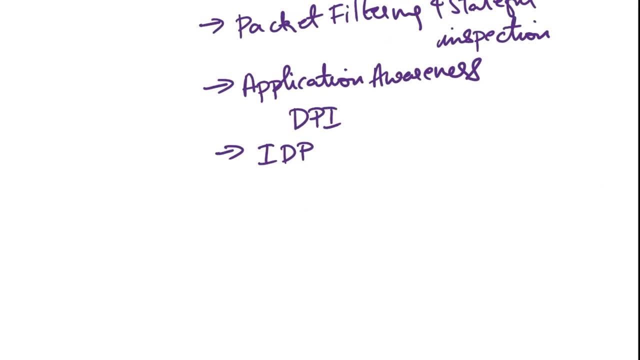 and prevention capabilities to detect and block suspicious or malicious network traffic. They use signature-based and behavior-based techniques to identify, verify and identify known and zero-day threats. Next characteristic is web filtering. Next generation firewalls can filter web content by inspecting URLs, webpages and web application traffic. This allows them to block access. 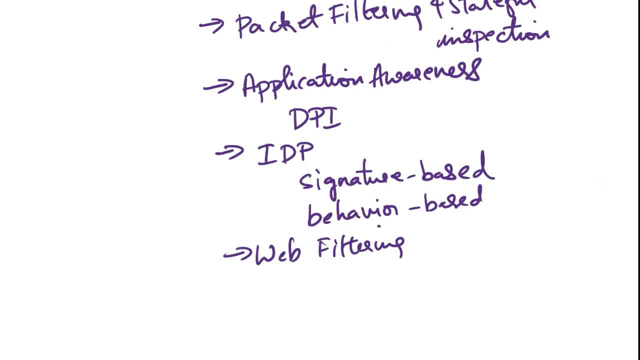 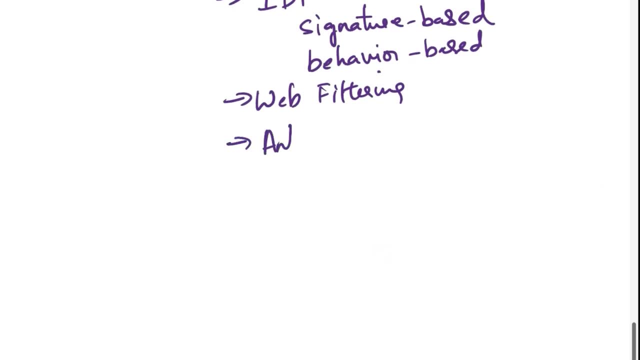 to malicious websites, enforcing content policies and protect against web-based threats like malware and phishing. Next is antivirus and antimalware. Many next generation firewalls, Antivirus and anti-malware scanning capabilities to inspect files and attachments for known malware signatures and behavior patterns. They can block or quarantine infected files to prevent. 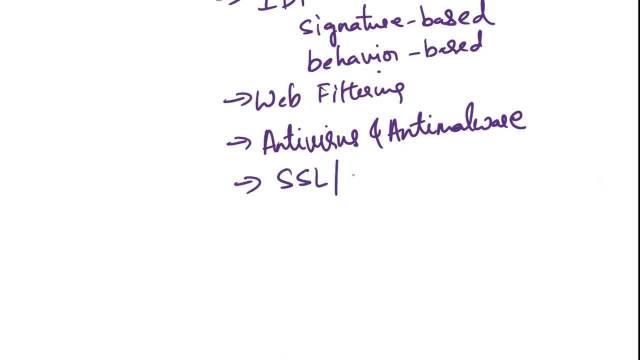 them from entering the network. Next is SSL and TLS inspection. Next generation firewalls can decrypt and then inspect the encrypted SSL TLS traffic to detect threats hidden within encrypted connections. This feature is crucial for identifying and blocking malicious activities in encrypted traffic. Next characteristic is advanced threat detection- Next generation. 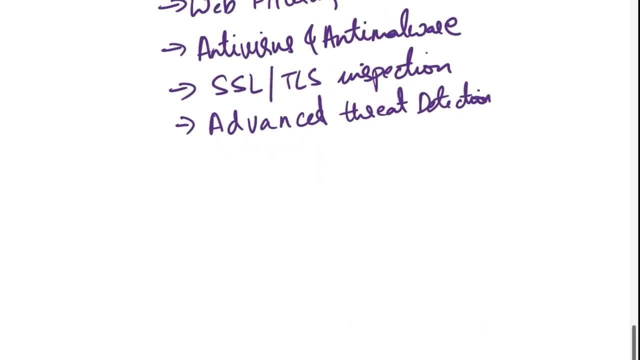 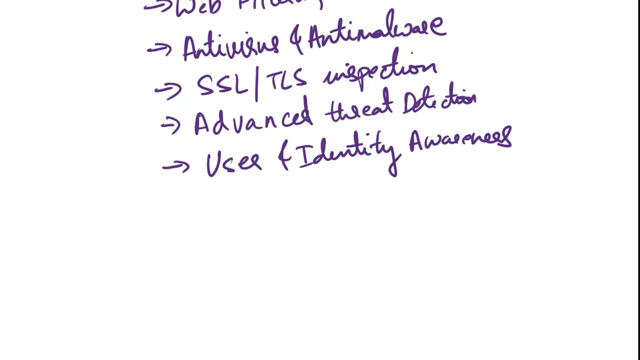 firewalls may incorporate advanced threat detection technologies, such as sandboxing and machine learning, to identify and mitigate previously unknown or sophisticated threats. Next is user and identity awareness. Next generation firewalls can integrate with authentication systems to associate network traffic with specific users or user groups. 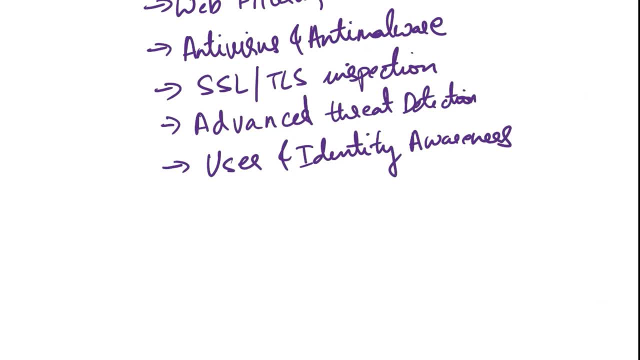 This allows for more precise access control and policy enforcement based on user identity. Next characteristic is application control, That is, in addition to identifying applications. next generation firewalls can control and prioritize application traffic based on business needs and security policies. Next is user and identity awareness, That is, in addition to identifying and utilizing. 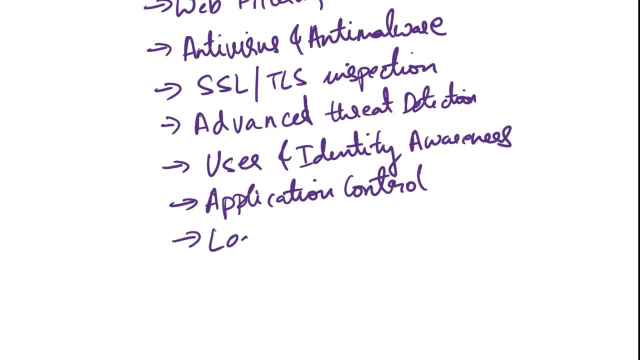 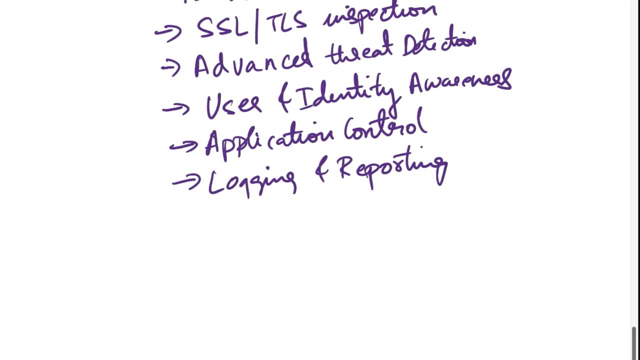 data, information and data for your organization. This helps organizations optimize network performance and protect critical applications. Next is logging and reporting. Next generation firewalls provide extensive logging and reporting capabilities allowing network administrators to monitor network activity, generate security reports and analyze incidents for forensic purposes. 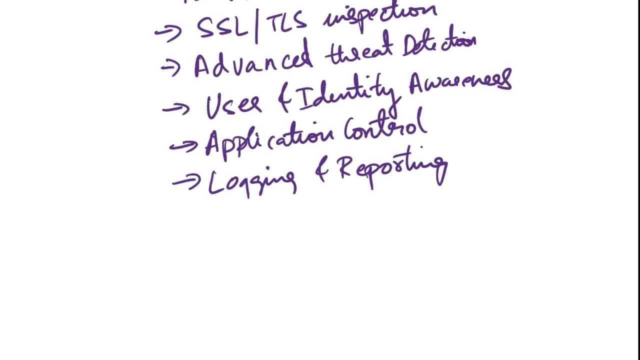 Next generation firewalls are highly versatile and are used in various processes to utilize data, various network environments, including corporate networks, data centers and cloud infrastructure. they play a crucial role in protecting against a wide range of cyber threats, ensuring compliance with security policies and maintaining network performance and availability. due to their 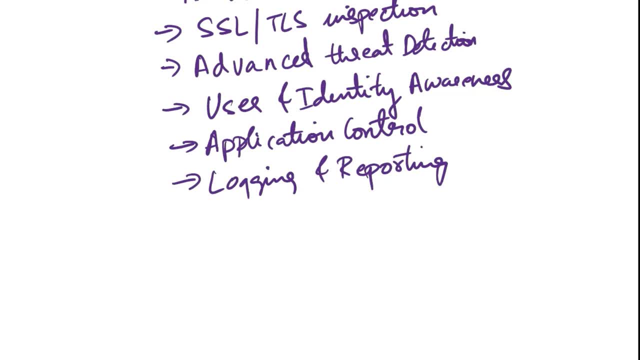 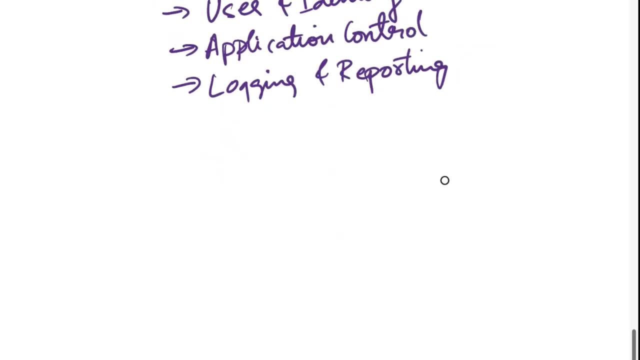 comprehensive security features. next generation firewalls are considered a fundamental component of modern cyber security strategies. the next firewall type we'll discuss is host based firewall, also sometimes known as personal firewall. it is a security software or component installed on an individual computer or host system to protect that specific host from unauthorized access network. 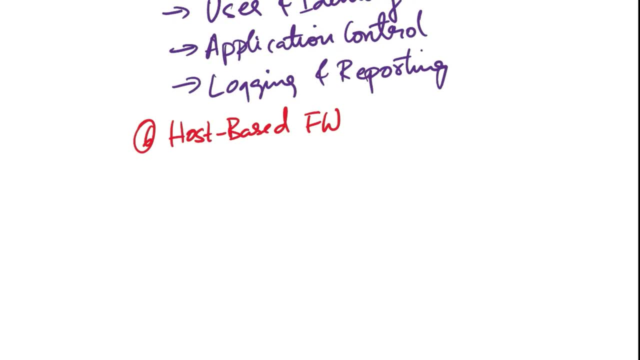 threats and malicious activities. unlike network level firewalls that operate at the network perimeter, host based firewalls are considered a fundamental component of modern cyber security. firewalls are designed to protect the host system itself, providing an additional layer of defense. let's see the characteristics. first is installation on host systems: post based firewalls. 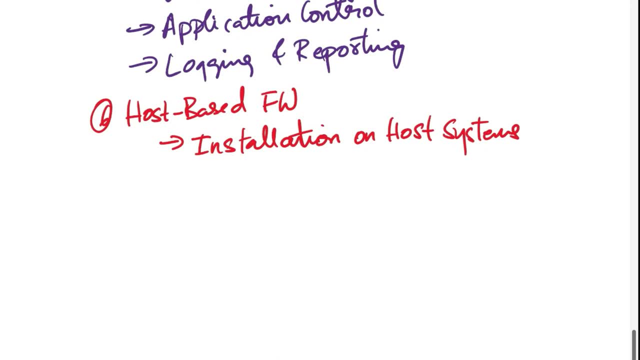 are installed directly on individual computers or devices such as servers, workstations, laptops or mobile devices. each host runs its firewall independently. next is packet filtering, host based. the firewalls perform a critical role in protecting the host system from unauthorized access network and to protect the host system from unauthorized access network and to protect the host system from. 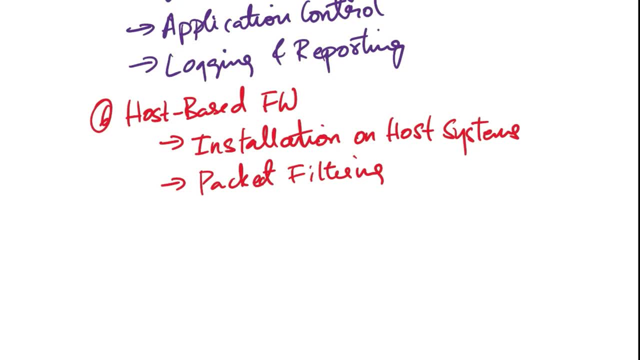 unauthorized access network. they perform packet filtering at the network layer, that is, layer 3, and transport layer, that is layer 4. they inspect incoming and outgoing network packets and apply pre-defined rules to determine whether to allow or block the traffic. these rules are typically based on criteria like source and destination, ip addresses, port numbers and protocols. next, 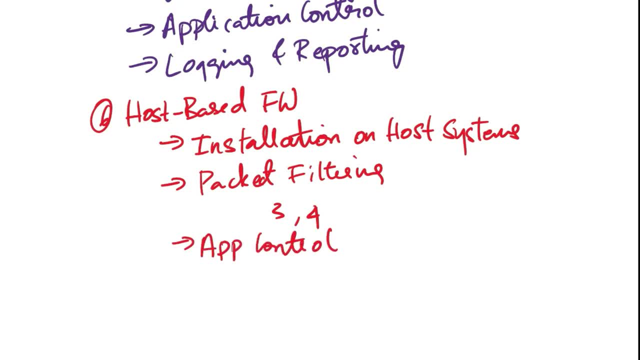 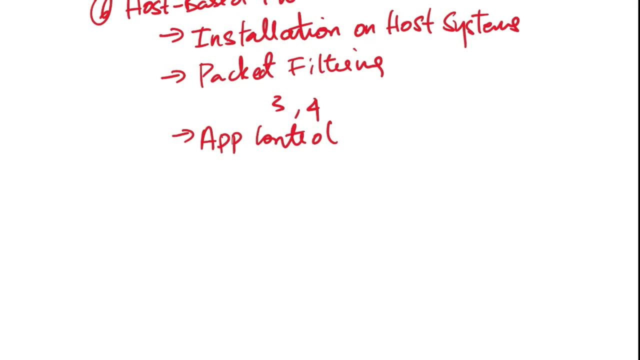 characteristic is application control. in addition to packet filtering, host based firewalls are can provide application level control. they can recognize specific applications or services running on the host and enforce access policies based on the applications themselves. this allows for granular control over which applications are allowed to access the network. next is stateful. 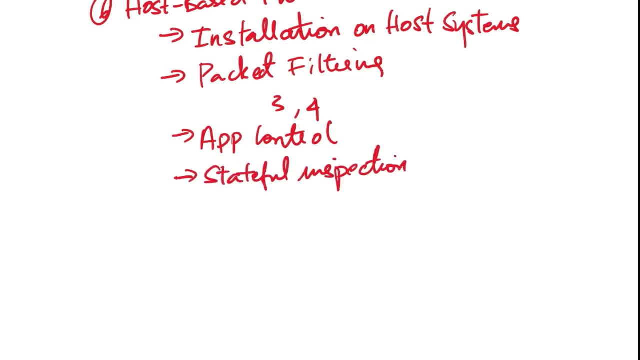 inspection. many host based firewalls employ stateful inspection, keeping track of the state of network connections and ensuring that incoming network connections are kept in good condition. and ensuring that incoming network connections are kept in good condition are part of legitimate, established connections. this enhances security by preventing malicious 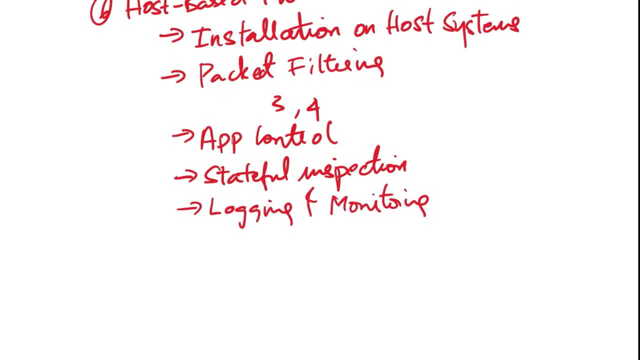 incoming traffic. next is logging and monitoring. host based firewalls maintain logs of network activities, including allowed and denied connections, blocked intrusion attempts and other security events. these logs are valuable for security monitoring and incident response. next is user and identity awareness. some host-based firewalls are part of the network activities and are part of the network. 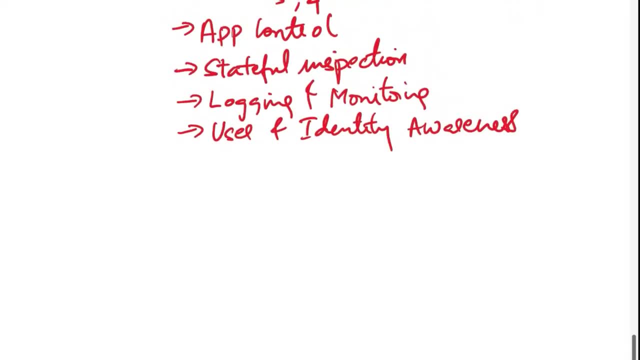 firewalls can integrate with user authentication systems associating network traffic with specific users or user groups. This allows for user-specific access control and monitoring. The next characteristic is customized security policies. Administrators can configure custom security policies on individual host systems to tailor the firewall's behavior to the specific needs. 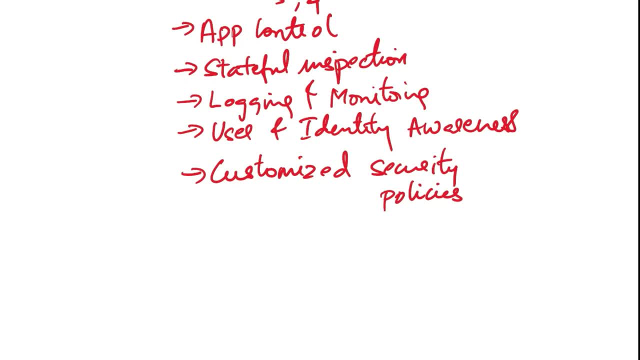 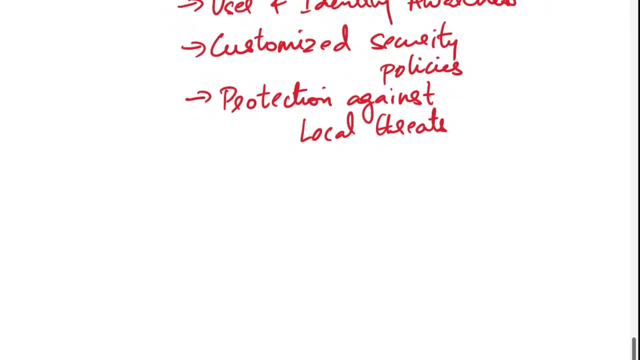 and security requirements of each host. This level of customization can be especially important in environments with diverse security needs. Next one is protection against local threats. Host-based firewalls not only protect against external threats, but also safeguard the host system from threats originating within the same network or system. Next is intrusion prevention. 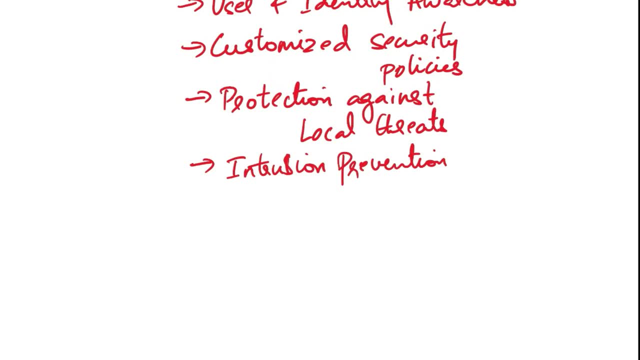 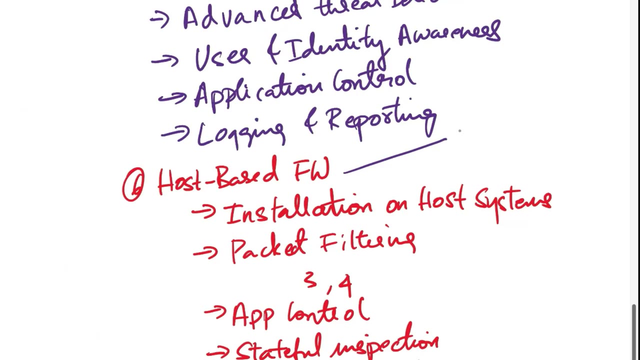 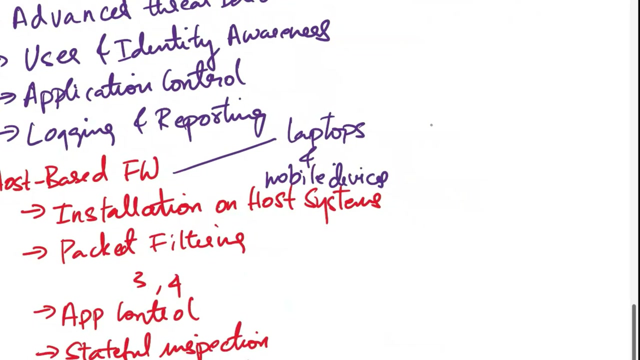 Some host-based firewalls include intrusion prevention features that can detect and block various forms of network-based attacks and suspicious behaviors at the host level. Let's see some of the use cases where host-based firewalls are commonly used. First is protecting laptops and mobile devices when connected to untrusted networks. Another use case is securing